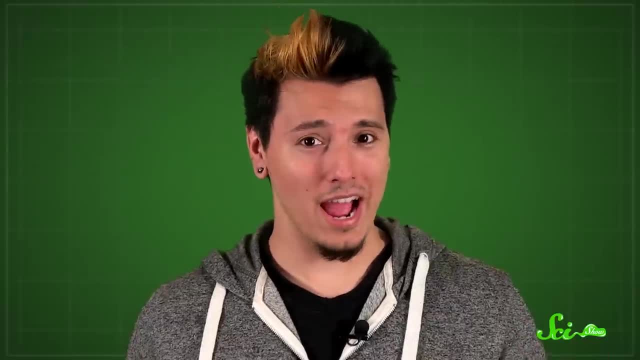 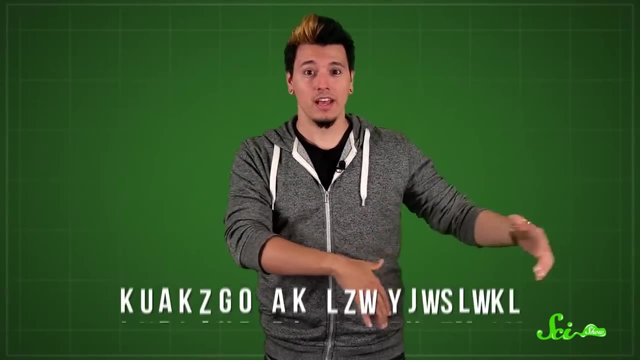 how many letters of the alphabet. I shifted it, But it's also very easy to crack, Even if you didn't know the key. it would take you at most 25 tries to decode the message, because you know that the whole alphabet has to be shifted by a certain amount. 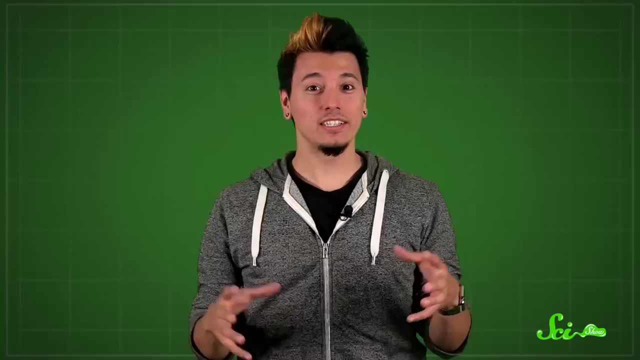 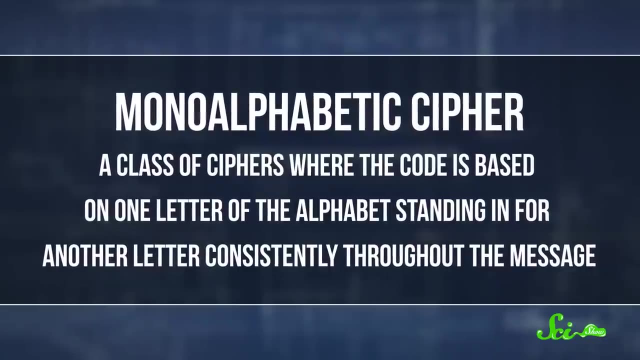 Since there are 26 letters in the alphabet, there are only 25 other options. A Caesar cipher is one simple type of mono-alphabetic cipher, a class of ciphers where the whole code is based on one letter of the alphabet standing in for another letter consistently. 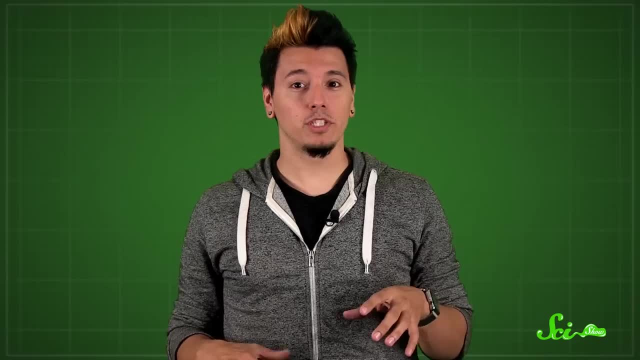 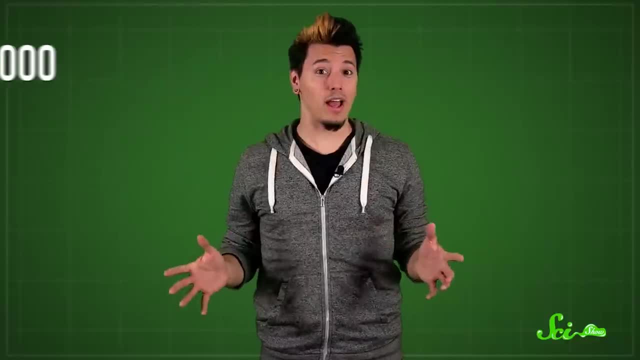 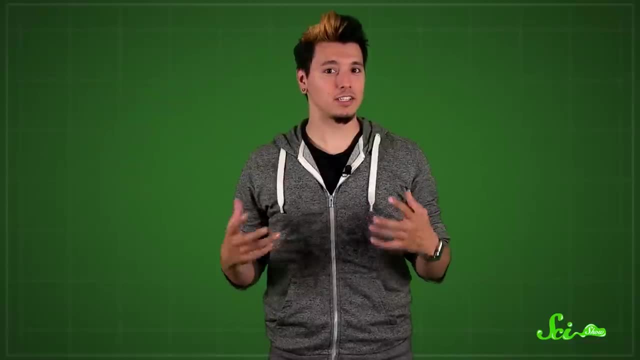 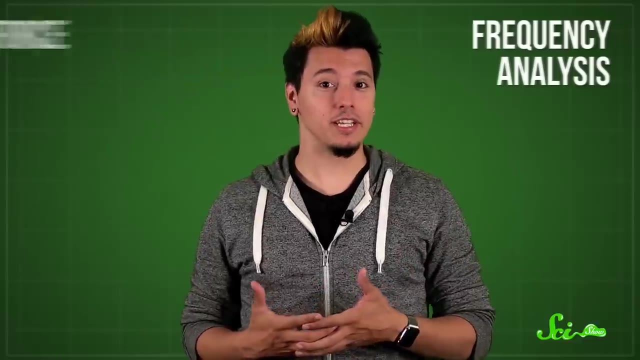 Just trying all the possible keys to a code is probably the most obvious and least subtle, and it has an equally unsubtle name: Brute force. But you can try a more sophisticated technique, something called frequency analysis, which is based on the idea that every language has its own specific patterns. 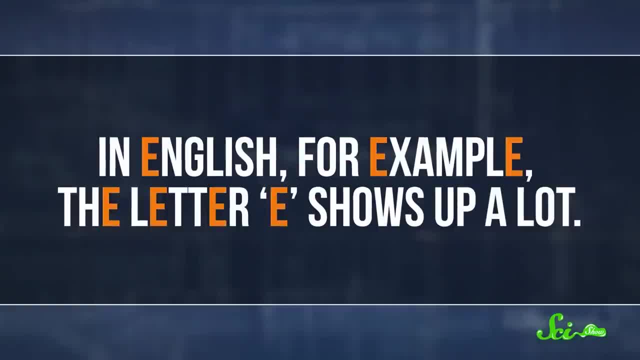 In English, for example, the letter E shows up a lot. I used it seven times in just the last sentence, And some words like the are so common that it's hard to understand. it's hard to even use a sentence without them. 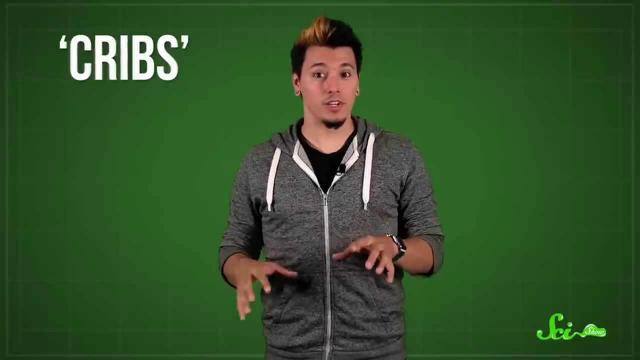 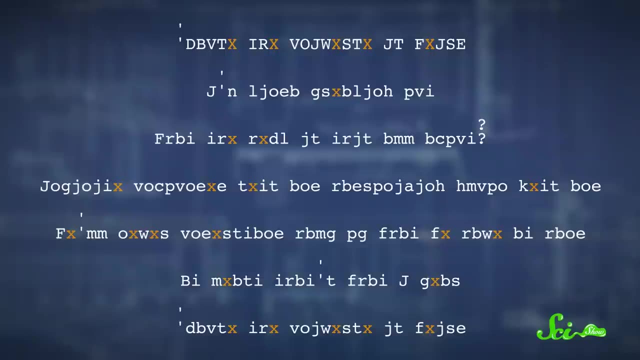 Cryptographers call these words cribs. So frequency analysis looks for common words and also common letters or sets of letters like E-D or I-N-G at the end of words, If you find that the letter X is showing up a lot in a message and so is the three-letter. 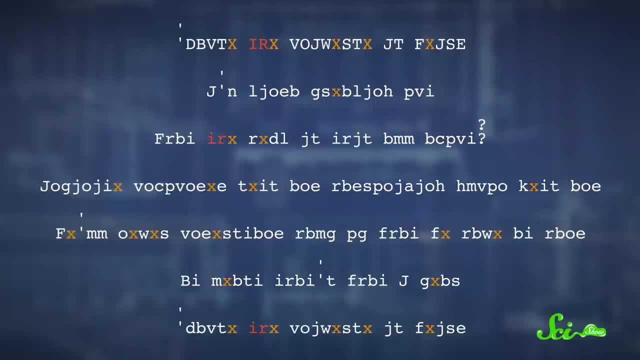 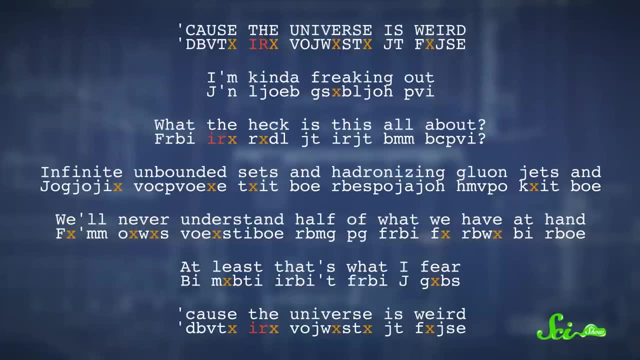 word I-R-X. you might guess that in the key X corresponds to the letter E and I-R-X spells THE. And once you've figured out those letters, you can figure out the rest by recognizing other words and using the process of elimination. 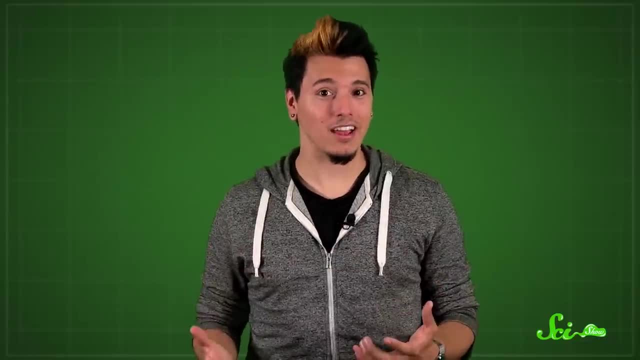 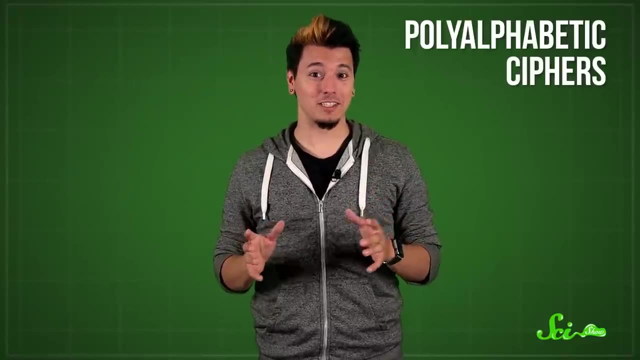 And since longer cryptograms contain more clues, they're easier to crack. So mono-alphabetic ciphers are fun, But they're not hard to break. If you want to get a little fancier with your encryption, you can use poly-alphabetic ciphers. 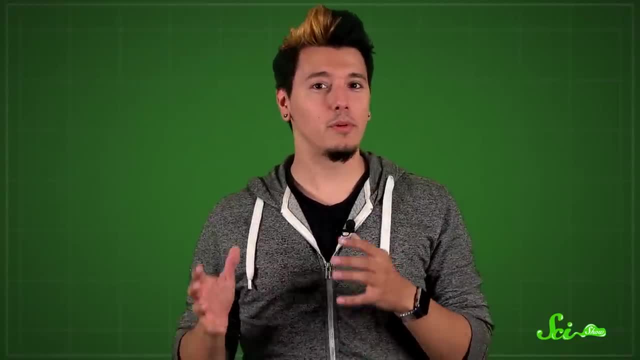 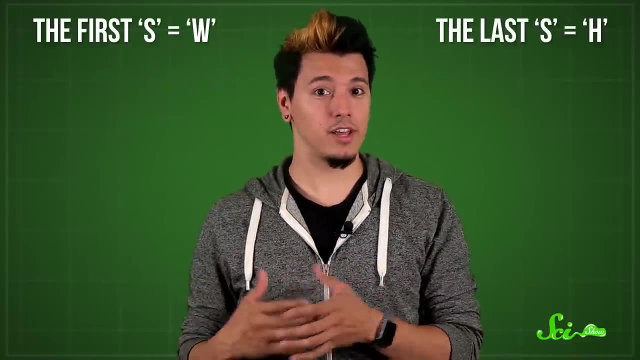 instead, They're much more effective. In a poly-alphabetic cipher, the way you scramble the alphabet actually changes throughout the message. In the first word, S might translate to W, But in the last word, S might translate to H. It all depends on the particular encryption method you're using and on your key. One of the earliest poly-alphabetic ciphers was the Vigeniere cipher, developed in the 16th century. It was pretty simple because the key was just a word. 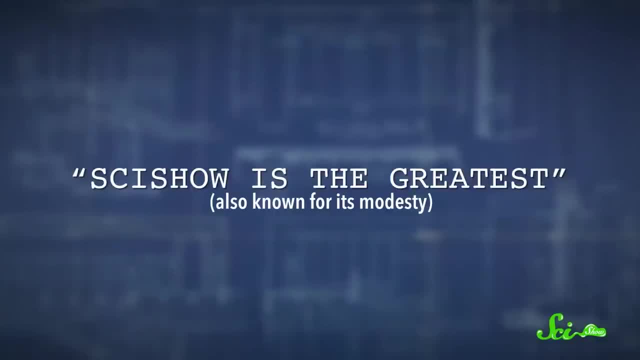 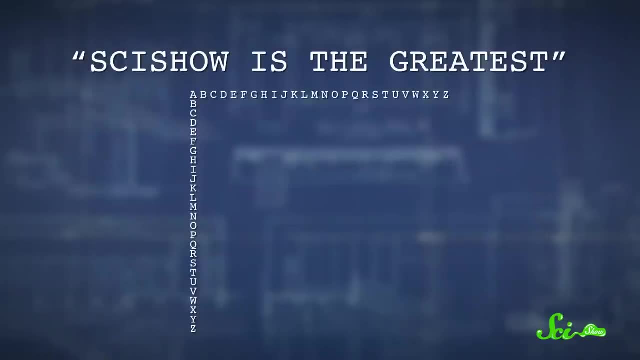 So let's say you want to encrypt- SciShow is the greatest- using a Vigeniere cipher. Well, the first thing you need to do is write out a Vigeniere square. The alphabet goes across the top and along the left side, and each row contains the letters. 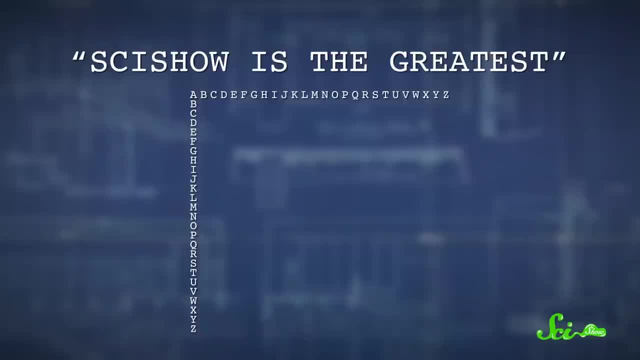 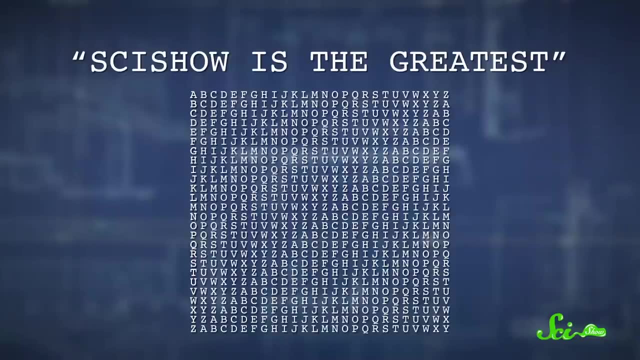 A to Z, shifted over by one. So the first line starts with A and ends with Z, but the second starts with B, goes all through the letters until Z and then ends with A, And so on. You end up with 26 differently scrambled alphabets. and now you're ready to encode the message. 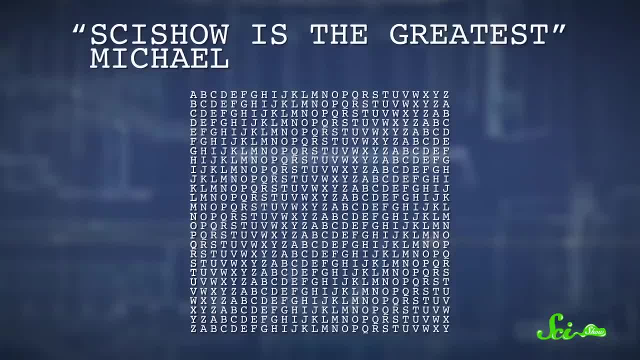 You just have to pick a key. Let's just say your key is Michael. You write out your key multiple times until it fills the same number of letters as your message. So SciShow is the greatest would correspond to this. Then, to encrypt it, you take each letter of the message and move along its row in the 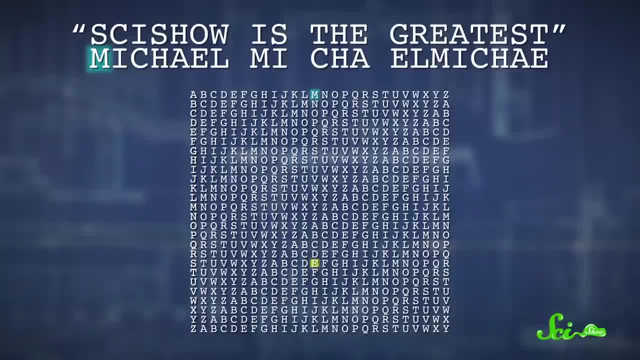 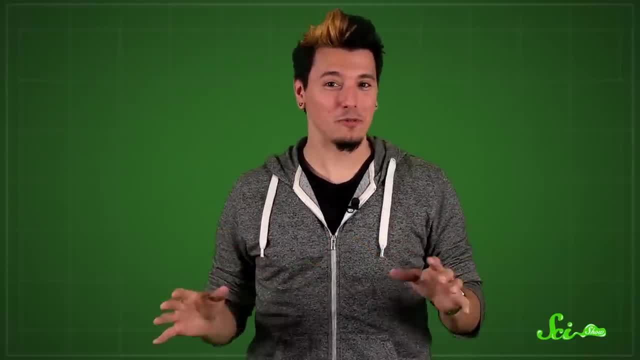 Vigeniere square until you get to the column of the corresponding letter in Michael. So SciShow is the greatest turns into this. That's much tougher to decode unless you have the key, because those letter frequencies are all different. now, Since the keyword Michael is seven letters long, each letter of your message is encrypted. 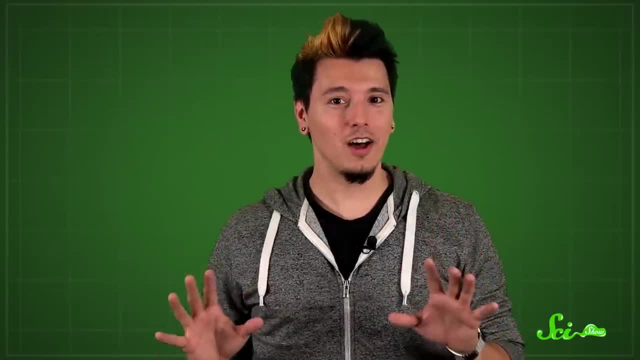 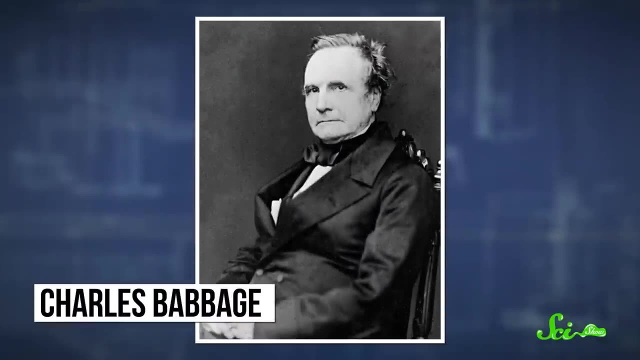 using seven different scrambled alphabets, But if your text is long enough, it's still crackable using a type of frequency analysis developed in the 19th century by cryptographer Charles Babbage. Babbage realized that in a long enough message, some patterns in the coded message will still. 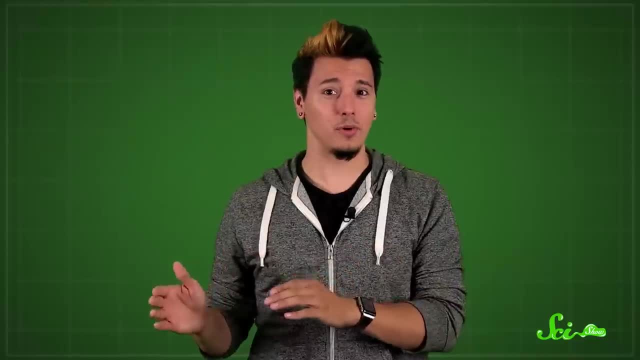 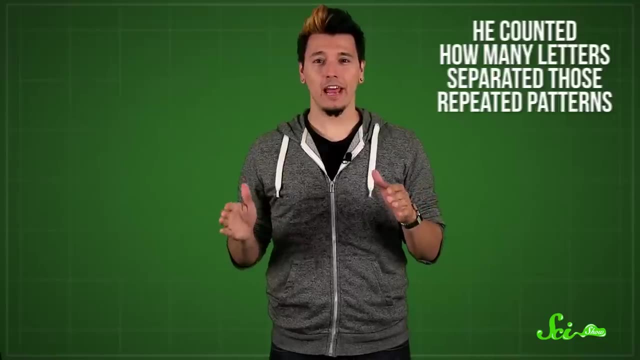 show up Like if your key only has seven letters. that means that there are only seven ways to encrypt the word the. But if your message uses the word the eight times, there are definitely going to be repeats. So he just counted how many letters separated those repeated patterns. 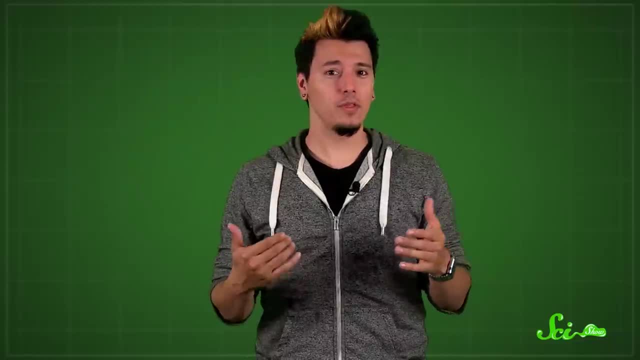 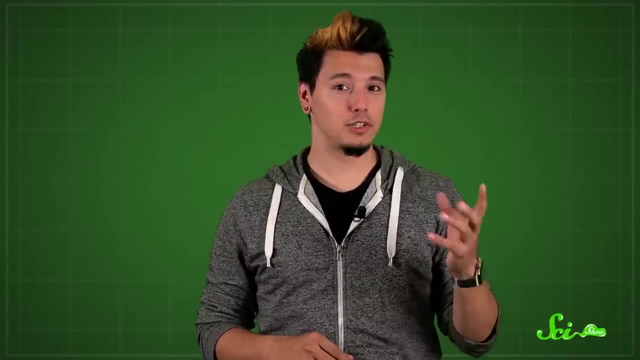 If they were separated by seven, fourteen or twenty-one letters. he knew that the key was probably seven letters long, And from there he would just use frequency analysis to figure out the seven scrambled alphabets. Babbage's method is just one example of why it's so hard to create an un-coded message. 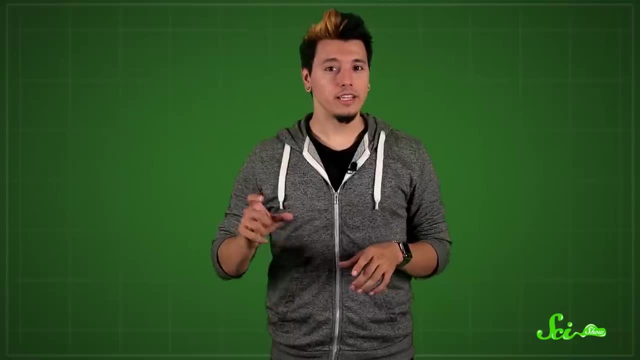 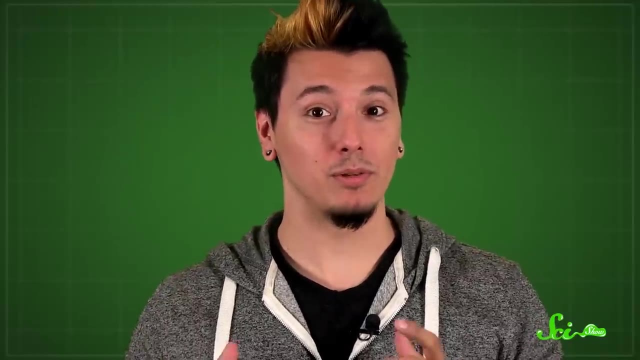 It's not just about the number of letters. It's about the number of letters. It's about the unbreakable cipher. Your key creates a pattern within the encrypted message and with enough work, a spy can uncover that pattern. It turns out that the only way to have a really unbreakable cipher is to use what's known. 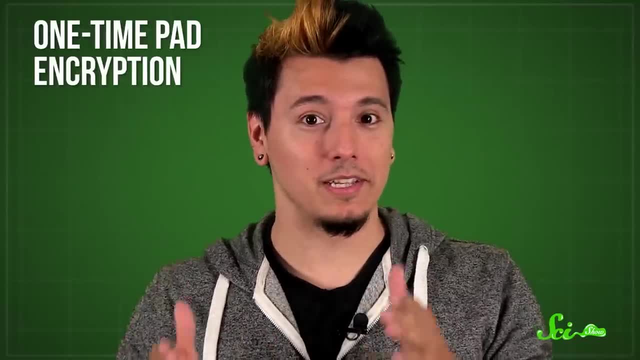 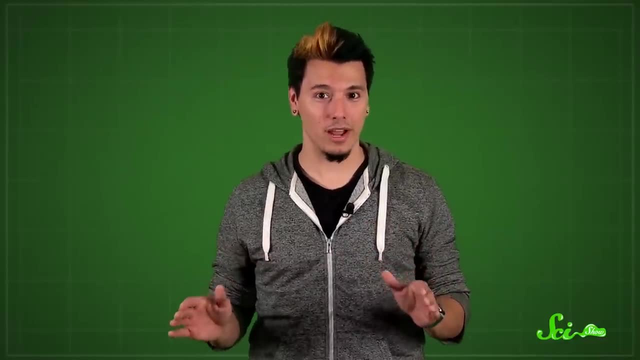 as a one-time pad encryption which uses a key that is as long as the message itself. That way, there aren't any patterns in the encrypted text. There's nothing to analyze, so there's no way to work backwards. The sender and the recipient both have the same pad and each sheet contains a long set. 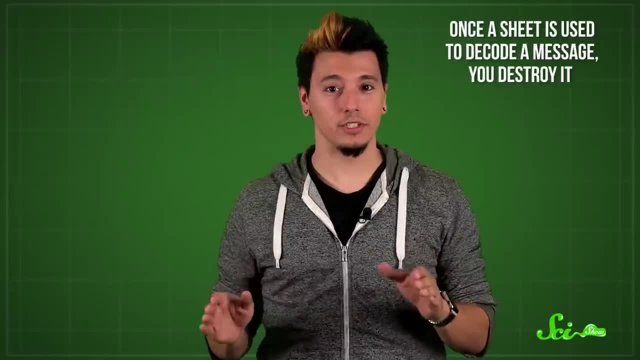 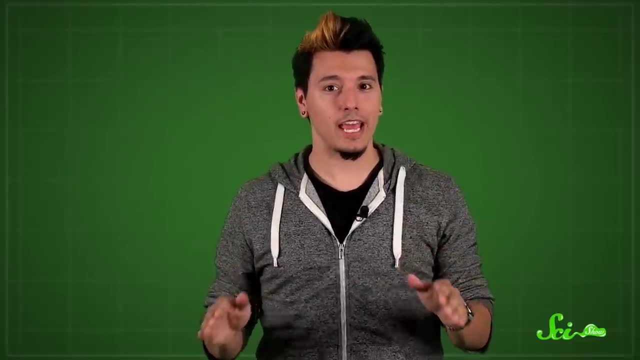 of random letters which is used as the key. Once a sheet is used to decode a message, you destroy it. Then you use the next sheet for the next message, so you never repeat a key. As long as you keep the pad safe, the message can't be decrypted by anyone else. 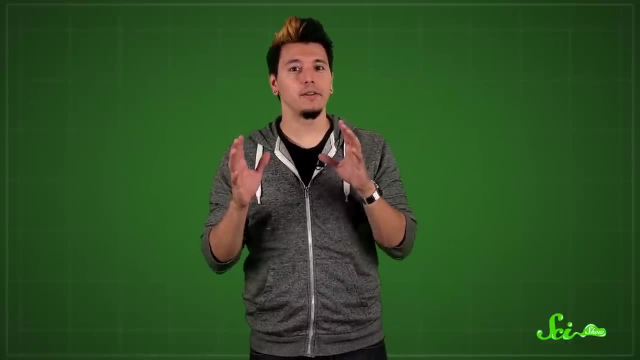 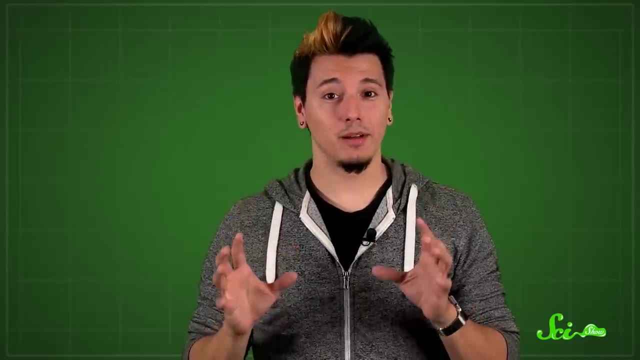 But you can't always use one-time pad encryption. Let's say you needed to get a message to someone halfway across the world whom you'd never met. You wouldn't have a chance to give them a matching pad. In warfare, that sort of situation comes up a lot, which is why in the early 20th century, 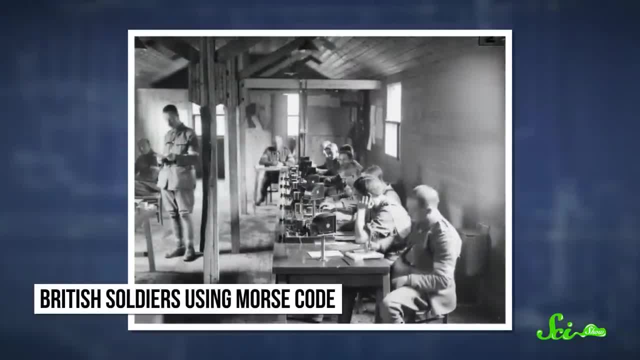 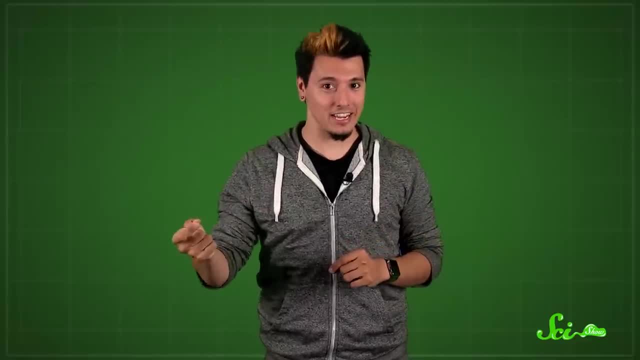 there was suddenly plenty of incentive to come up with better ciphers. Remote communication using technology like the telegraph was incredibly valuable during wartime, But it was essential that only your allies understood what you were saying. The Germans experimented with a new, more complicated mono-alphabetic cipher during World. 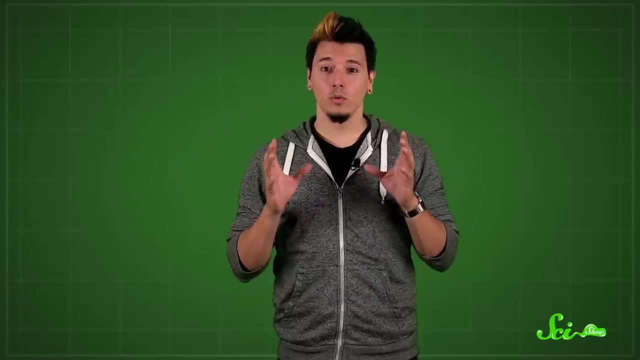 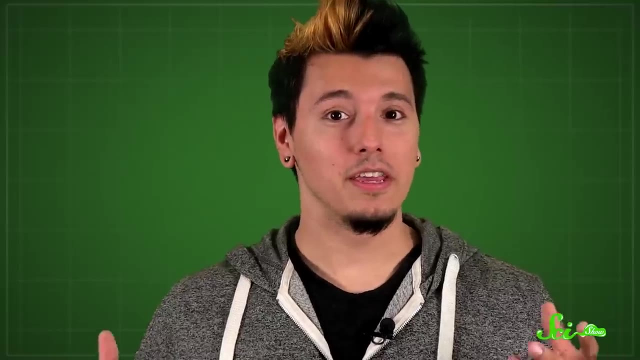 War I, But eventually the French managed to crack it. Then, during World War II, the Germans again came up with a new cipher, And this time its security seemed perfect. Maybe you've heard of it: The Enigma machine. 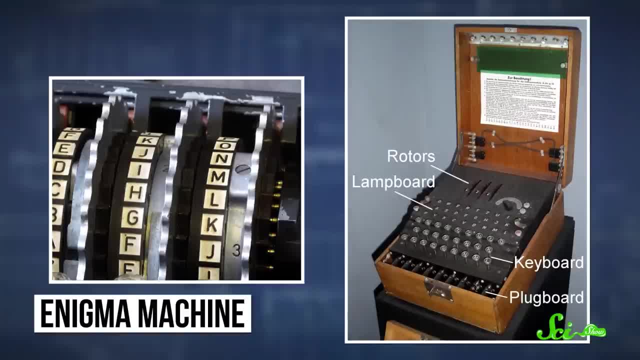 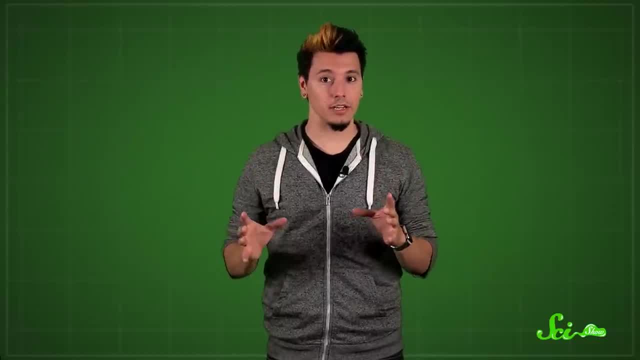 The machine used a poly-alphabetic cipher that scrambled the alphabet in a different way each time you typed a new letter. As far as the Germans knew, the only way to decipher the message was to have your own Enigma machine and set it up using a secret key that changed everything. 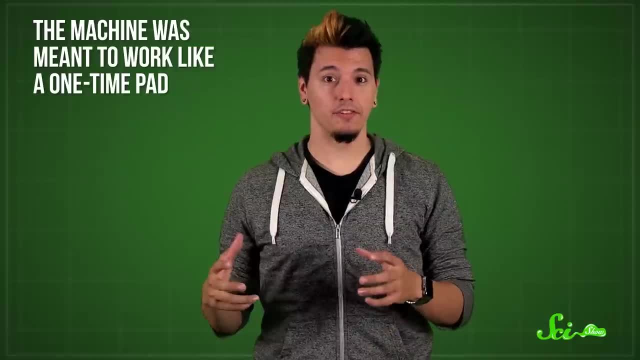 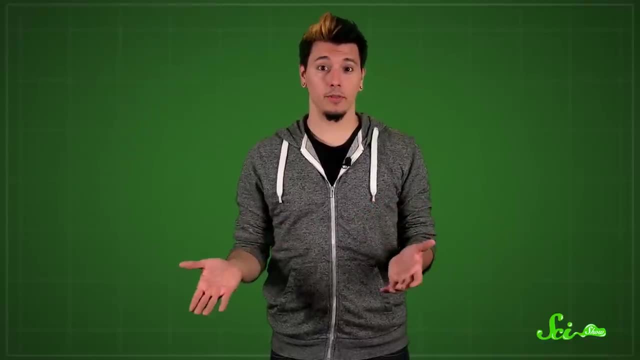 Every day. The machine was meant to work like a one-time pad, in the sense that the alphabet was re-scrambled for every letter of the message, But instead of having to distribute a set of sheets to everyone, you could just use a key that told the users how to set up their Enigma machines. 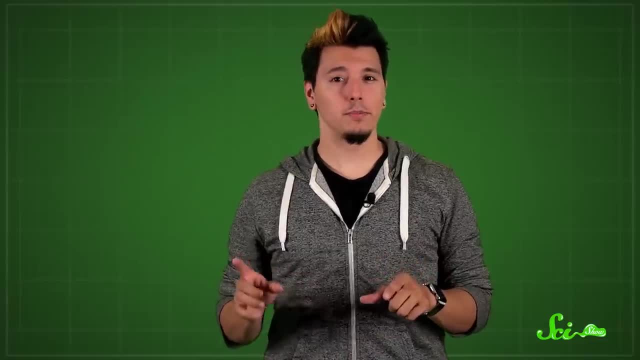 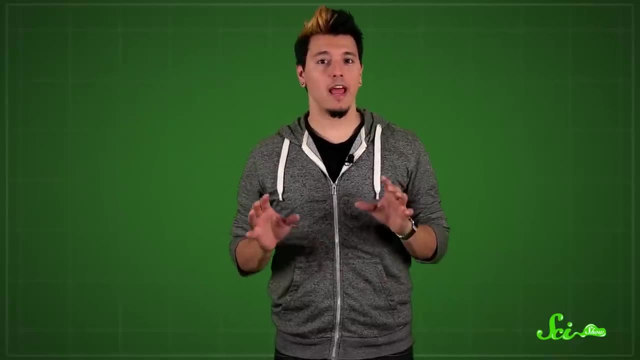 And you could change that key as often as you wanted. But it had a few flaws. For example, no letter could be encoded as itself. That might not sound like a big deal, but it ended up being a fatal weakness. British mathematician Alan Turing, along with the rest of his team, designed a machine of 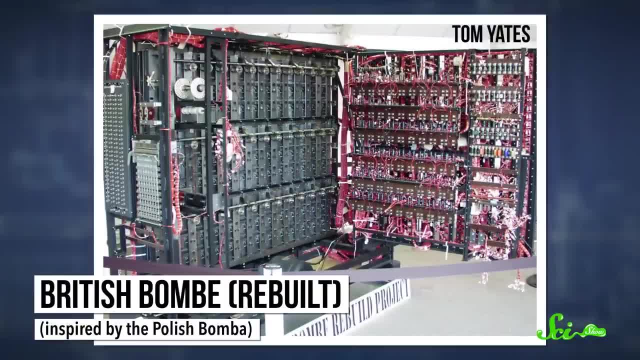 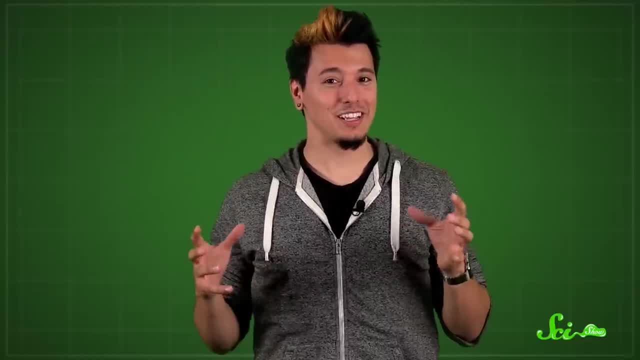 their own that could crack the Enigma code, as long as they knew around twenty of the characters contained in the message, Which they often did, because some phrases tended to show up a lot in Nazi communiques, especially nice things about Hitler. So part of the strategy of Turing's team was to look for cribs, those common words. 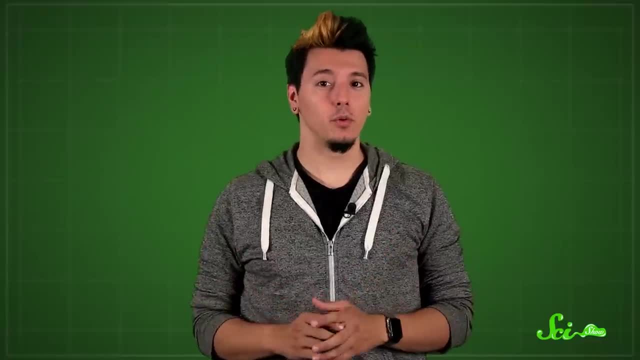 and phrases and see where they might fit. For instance, if they knew a message contained the word Führer, they could look for places in the text that didn't have the letter F, since they knew that the F in Führer couldn't. 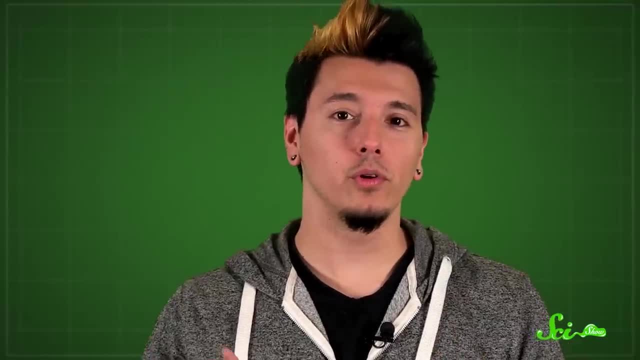 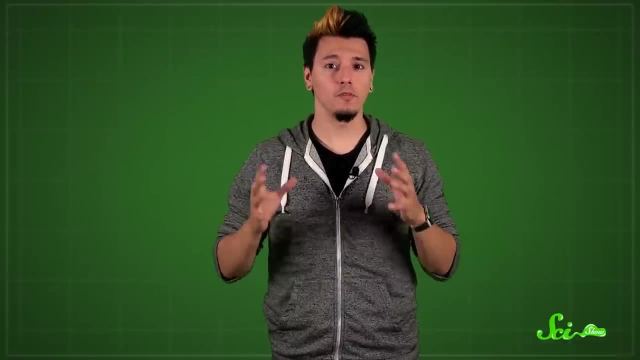 be encoded as itself. Those clues helped them figure out how the Enigma rotors were set up to encrypt the message. Cracking the Enigma code was a huge advantage for the Allies. Many historians attribute some of the most important victories during the war to information.